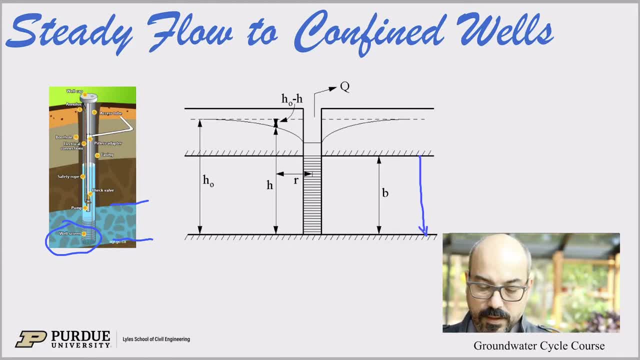 have a potentiometric surface, meaning their depth, here B does not change, right, the depth doesn't change because, again, since they're confined, since they're confined, there's no, you know, dipping of the actual water level. the water level is constant. What changes is the head? 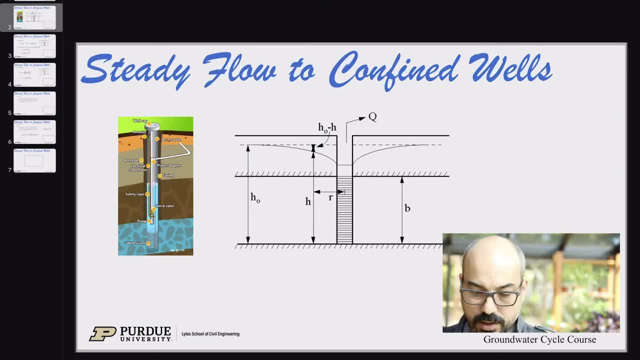 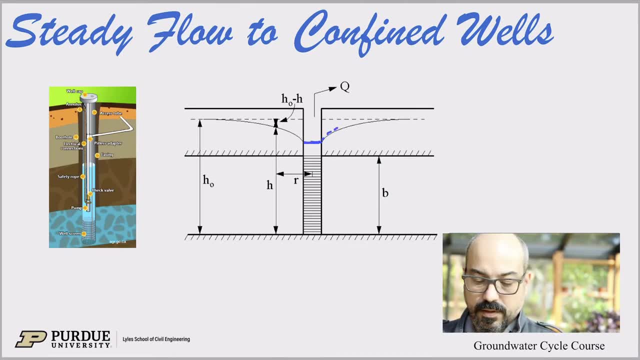 in the water, right? so when you're pumping it, what you change- and I'm sorry, this always does that- so when you're pumping it, what you change is the potentiometric surface here. So again, imagine this is your steady water level or, excuse me, this is your steady water level when you're not pumping. 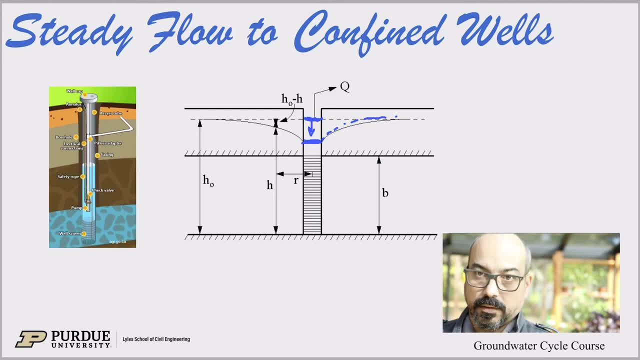 When you start pumping, obviously the water level drops in the well and with it, with the water drop in the well, what drops is the head, basically, or the potential surface. okay, So the potential surface, you know, if there's no pumping, is somewhere here. so again, assumption of flat and stable and 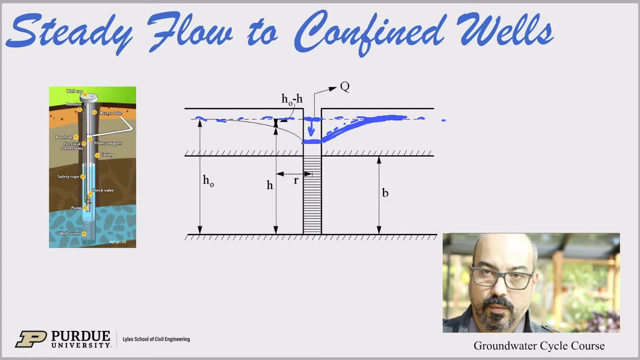 everything. and then, when you start pumping, you're dropping the actual water in the well, but you're not dropping water in the aquifer, you're dropping the potentiometric surface. Okay, so you can see that the water is going to rush into the well from left and right, from. 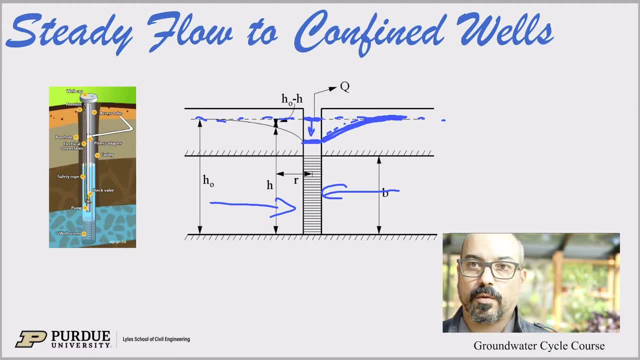 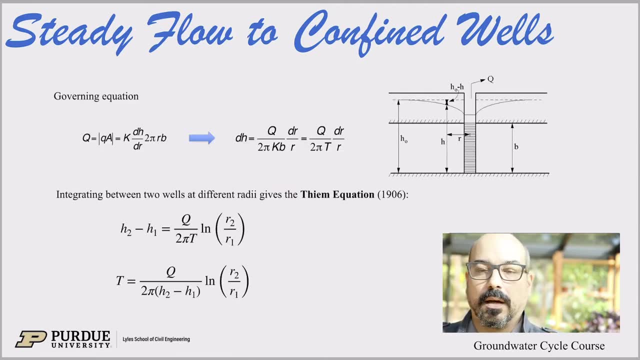 everywhere radial coordinates from all around that. well, Let's look at these equations. Okay, so we start where we always start, which is essentially a continuity statement. right, We're saying that whatever water you pump out of the well must come from somewhere. right must be. 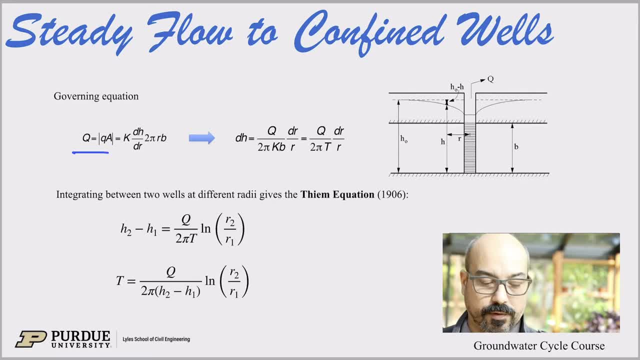 equilibrated by flowing to the well from the aquifer. So we can say that. so the flow into the well from the aquifer is the Darcy flux times the area. Again, if you didn't take the first course, I'm sorry, but you should really go back and take a look at those lectures and you'll be able to see. 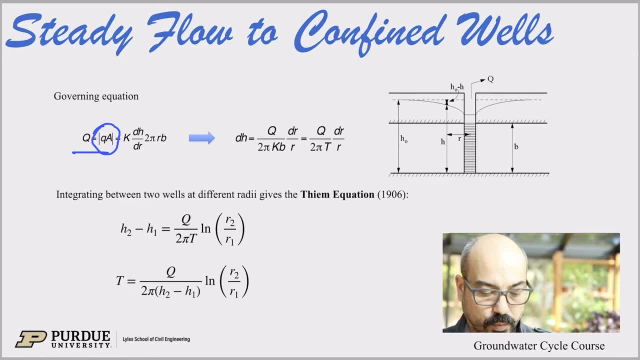 on Darcy's law. So then when we write the Darcy flux as Darcy's law, so k a hydraulic conductivity times the hydraulic gradient, and again now we're in radial coordinate right. so it's dh dr, right? this is your Darcy's law. for you know, when you replace: 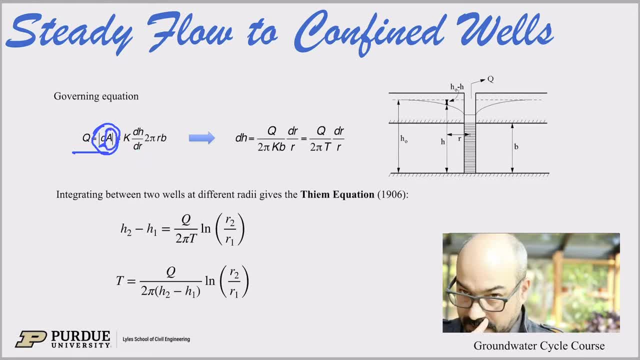 x with r And then the area here. so this is where the trick is important to understand This area. here is the area through which the water rushes into the well meaning. this is the area of the casing here, all the way around the screening right. So this is the area of 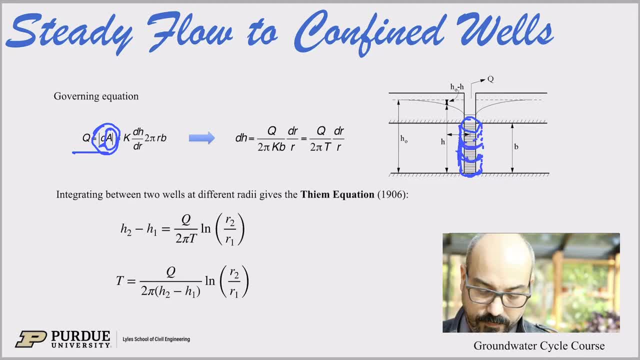 that cylinder right. There's a cylinder here where the water comes in from all around. So the area we're looking for is that area all around the well, where the water is seeping into the well, where that screen was in the previous picture. 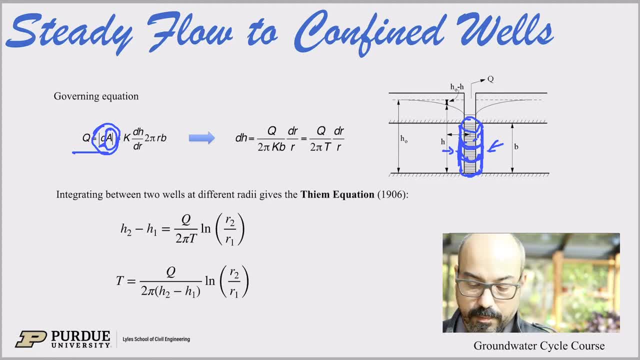 if you will. Now, the area of this is, of course, the perimeter times the height of the cylinder. so it's two pi r for the perimeter at the top and then B for the size you know down. So this is the area around that sleeve, if you want. 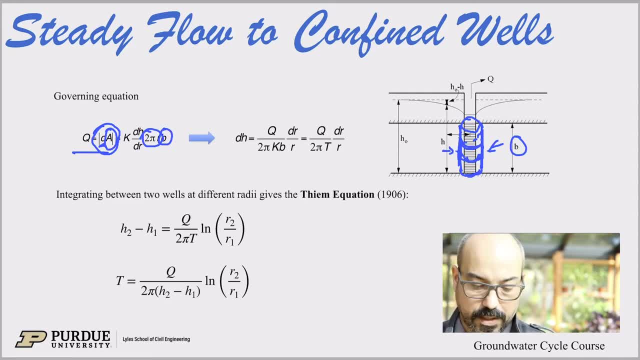 around the well where that water is seeping in. If you understand this, you understand most of what you need. Okay, so now, once we have this equation- and I'm sorry, I'm just cleaning up a bit here- Now that we have this expression, we can just do the usual mathematical trick. 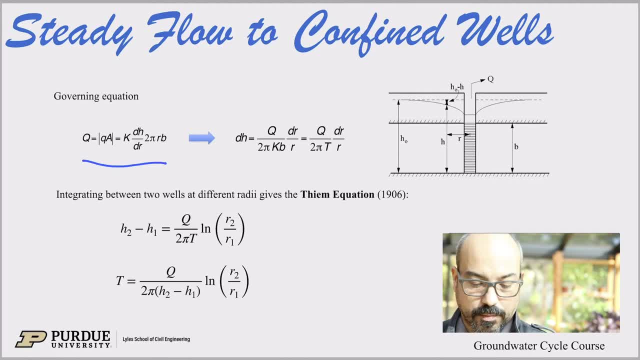 where we separate the variables right and then we integrate. So, separating the variables, we get dh on one side and then 1 over r, dr on the other side, And then everything else is some constants that we bunch together here, right. 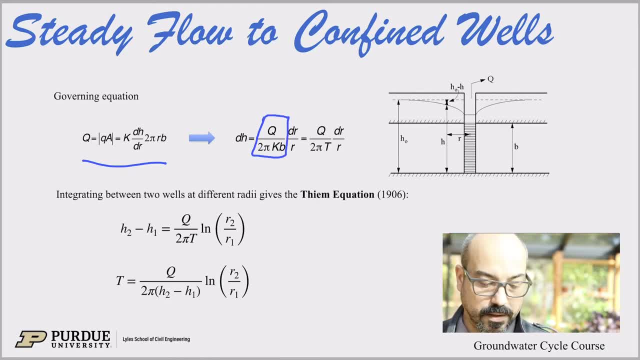 So we have some constants right: the hydraulic conductivity, the depth of the aquifer b, the pumping rate, q, right? These are all known numbers, if you will. And then we separate the variables, which are again 1 over r, dr and then dh on the left-hand side. 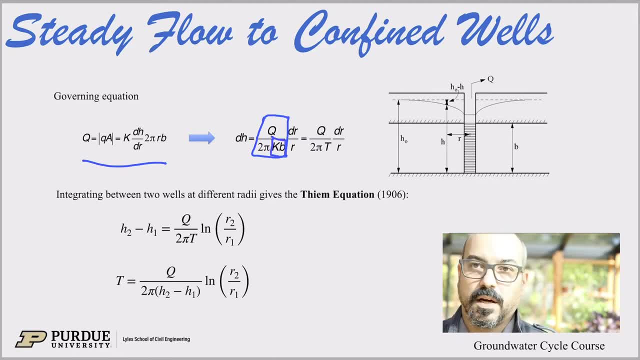 Remember that kb is the transmissivity of the aquifer, and that's typically what we want to know when we do Wells tests or aquifer tests. So we can replace kb with t and this is the final expression. Now we can put an integral on both sides and solve. 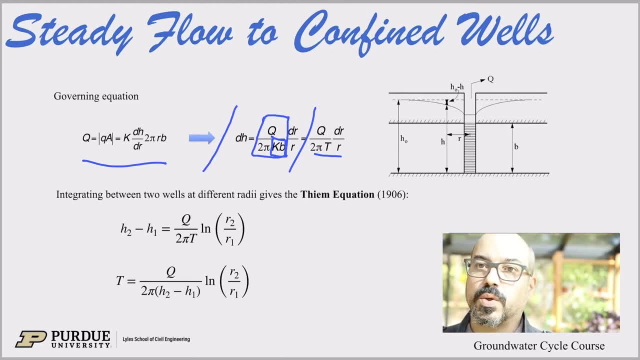 So obviously 1 over r, dr is going to integrate to the natural log right ln. So you know, integral of 1 over x is lnx. So we do that. and then the integral of dh obviously is just h between. you know the two points. 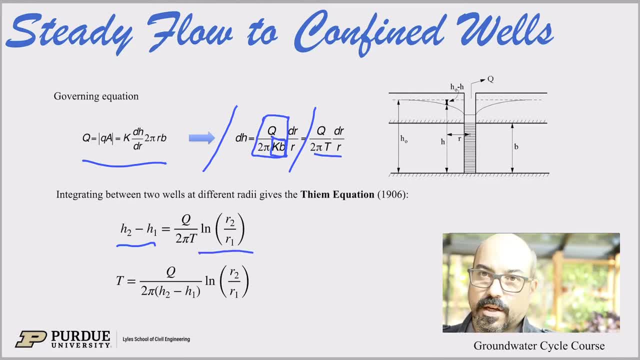 So now we get h between two points, natural log of r between two points. Again, remember that r2 minus r1 equals the ratio, right, just by mathematical rules. So then, this is it. Now we have an equation Where we can, for example, find the transmissivity from two points, right. 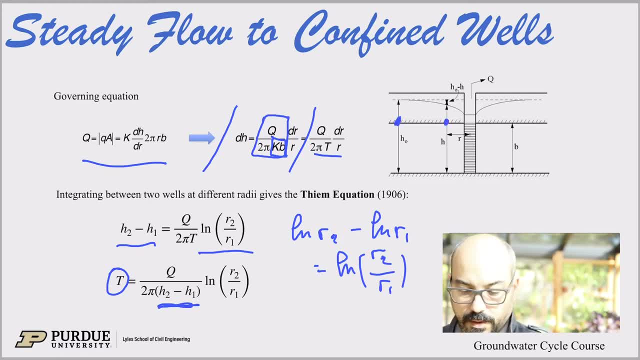 So if we have two points at different distances from our well, here let's call this h2 and h1, here and here, If we can measure two points with two observation wells at some distance from our pumping, well now we can actually calculate, for example, the transmissivity of our aquifer. 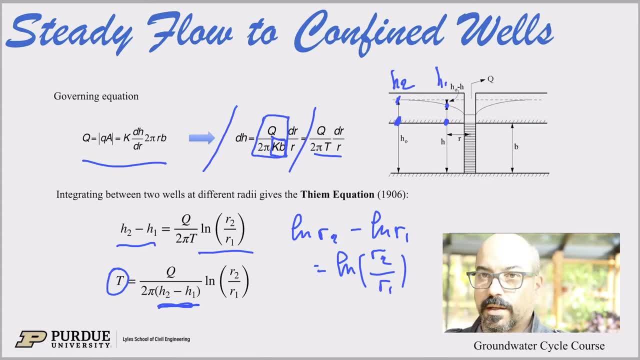 which is typically what we want to know for water resources. right, How much water can we get? So again, remember, transmissivity is a normal, It's a normalized flow. basically, It's how much water can that aquifer give us per unit of head drop right or per pumping? 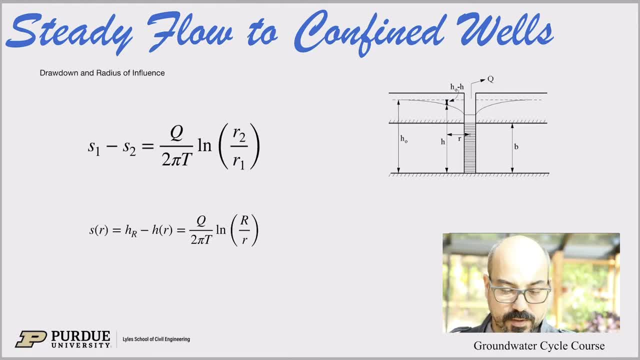 Okay. so how do we use that? I'll just do a quick, simple example. Oh, one. before I do the example, one, quick introduction of drawdown. So the drawdown and the radius of influence, these are two important concepts. 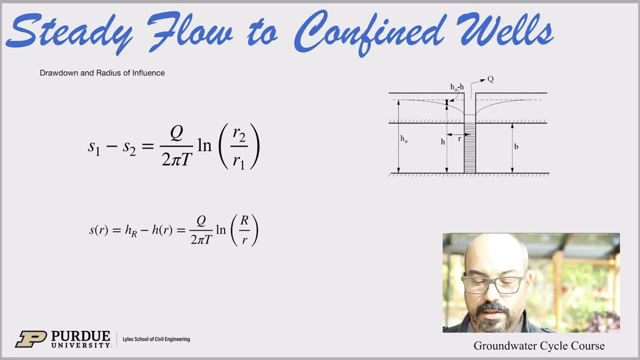 So the drawdown is basically like the head difference, but it's really the water missing at the top. So the drawdown here is h0 minus h. So the drawdown is really, you know, the amount of water that you pumped in the well. 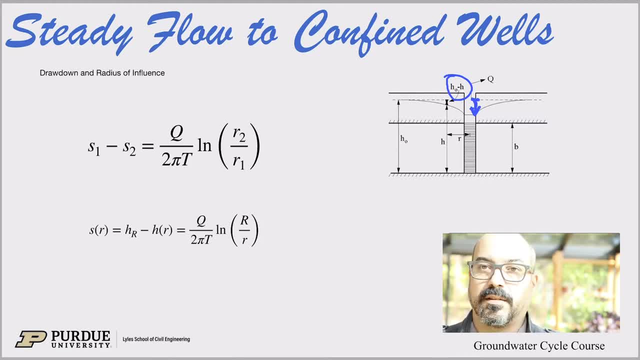 So the drawdown in the well is literally the difference between the stable level, when you don't pump, and you know some level later. So that's the drawdown And this is different from because, again, when we do head right, the head is the height of the water. 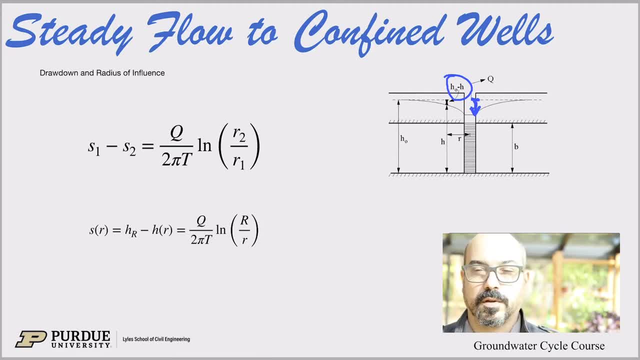 or you know, for an unconfined case it's the height of water, For a confined case it's just The potentiometric surface here, but it reflects the height from some datum, from the bottom of the aquifer, basically. 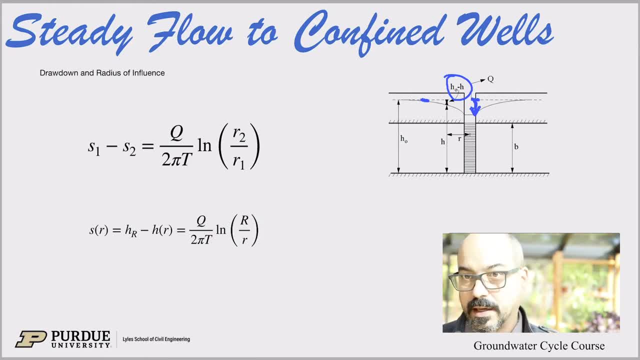 But typically when we pump we don't know where the bottom is, or we might not know where the bottom is. What we do know is where that you know water surface is, or that water in the well. that's easy to measure, right. 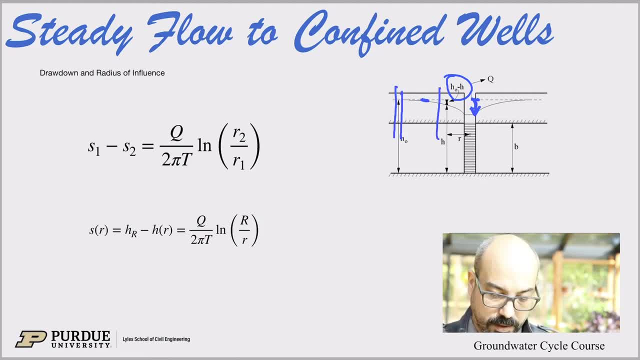 So if you again, if you do a couple piezometers here and here, right, the water here and the water here, you can measure this easily, and the water here, you can measure this easily, And so it's easier to quantify. 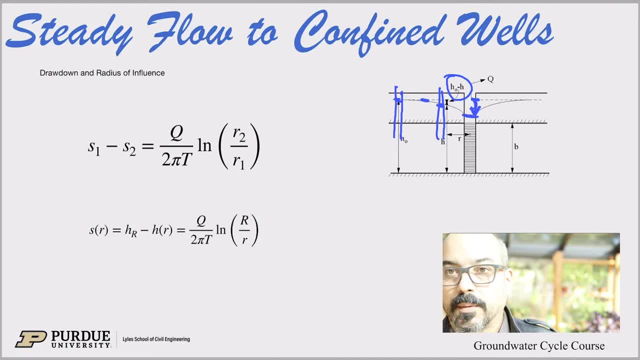 So if we convert everything into drawdowns, so meaning you know depth of depth to the water, as opposed to you know depth of water from some bottom that you don't know where it is. So again, it's basically the same right, but it's just inverted. 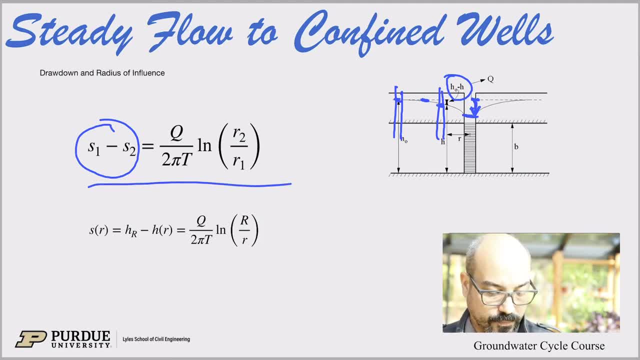 So now you can write that same equation as before. you know again, with the drawdown being the difference in head, you know from some point to another point. Now, if we write the drawdown as a function of distance, right? 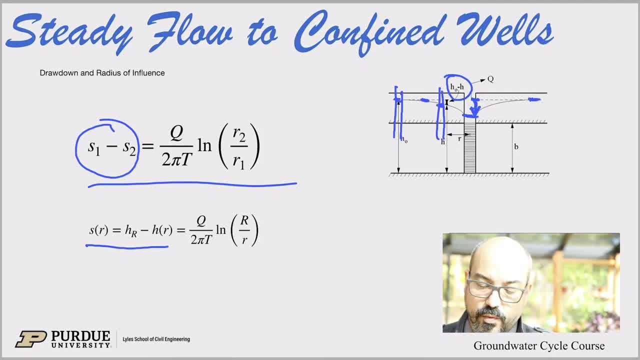 we can say that it is so. if we take, basically so, the radius of influence, if we take a point where the influence of the well is zero, basically so, there's no more influence of the well on the, either water table or, in this case, 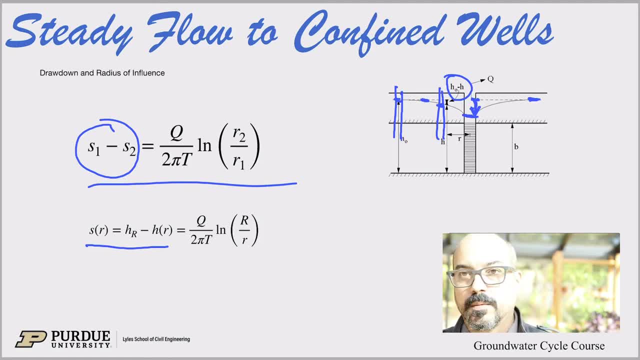 on the potentiometric surface for a confined case right. So at some point far from the well, the pumping has no influence, like there's no drawdown. basically Drawdown is zero. So that's what we call the radius of influence. 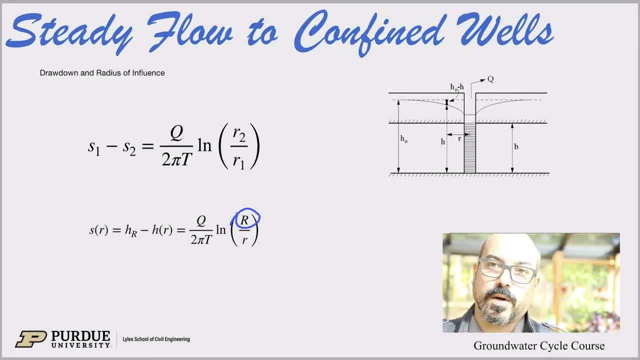 So the radius of influence. here again, if you have an observation, well, that is sufficiently far from the well. there's a point where, basically, the well has no influence on the potentiometric surface, and that's the radius of influence of the well. 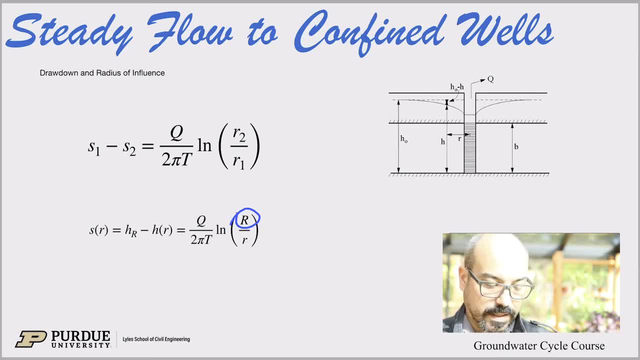 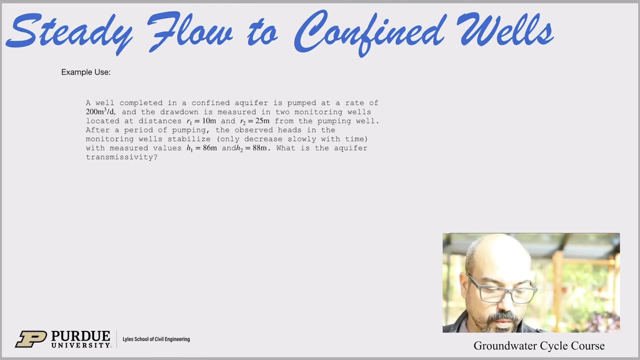 And again, you can solve for this by setting your drawdown equals zero. Okay, so we'll do many examples of that, but this becomes pretty important, Okay, so here's our quick example to wrap this up. So a well is completed in a confined case. 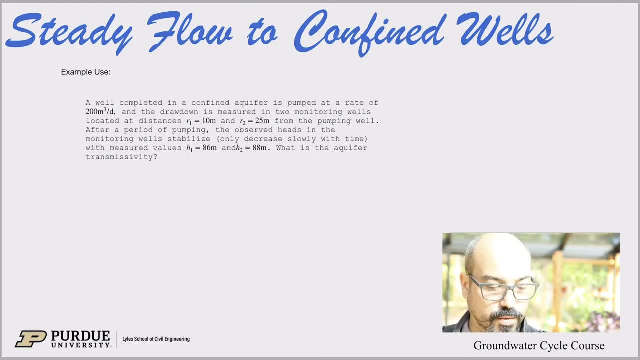 So a well is completed in a confined aquifer and pumped at some discharge- Q 200 cubic meters per day. The drawdown is measured at two monitoring wells which are 10 and 25 meters from the pumping well. So now we have those two observation wells, 10 and 25 meters from a well. 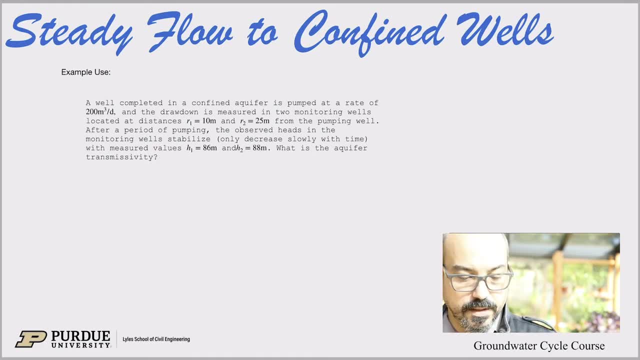 The heads in the monitoring well stabilize, and they're measured at 86 meters and 82 meters in those two wells. So again, remember that These are not given in heads, not in drawdowns right, So they're given as the depth of water seen into those observation wells.